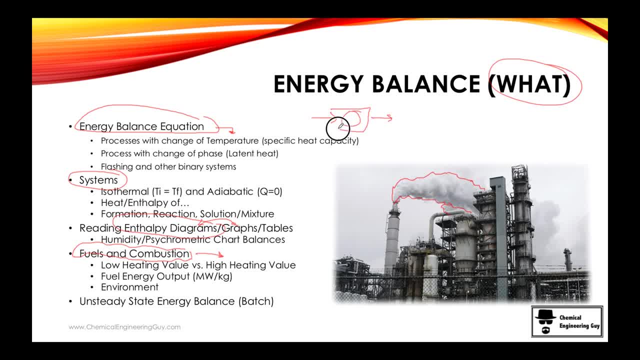 Efficiency, Efficiency, Energyomy. there's a lot of parallel things. right, we have to start on like Efficiency, Energyomy. Finally, not everything is going the way we'd like. First thing, iri 80 celsius. so the first thing we do is: how do we change temperature? what's the specific heat? 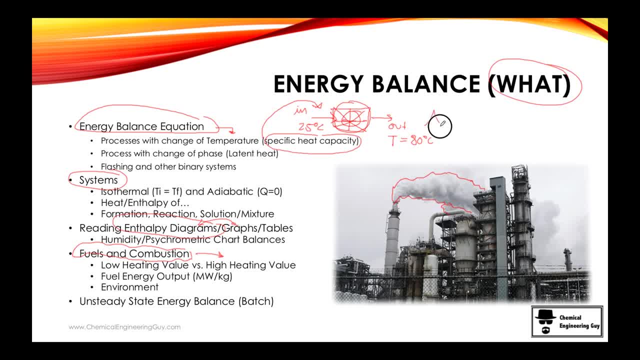 what do we use? eventually, we're going to understand that there is a change on enthalpy. now this is typically for a pressure which is constant, constant pressure. we're going to work in general with constant pressure all the way down now, eventually, guys, you know evaporators. 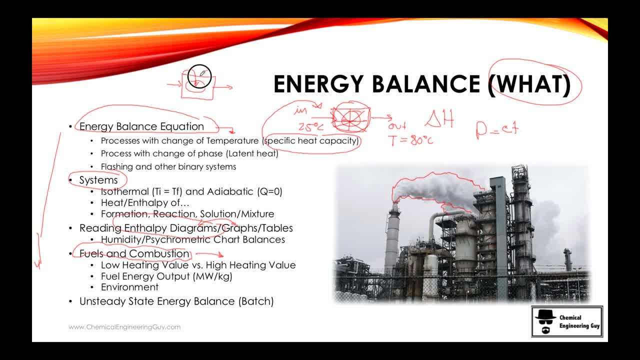 we don't know how they work inside, but we do know that if we have water at one atmosphere and we bring it at 25 celsius and we heat it up to 110 celsius, we're going to have vapor because there is evaporation. this is called latent heat or, using the energy equation, with 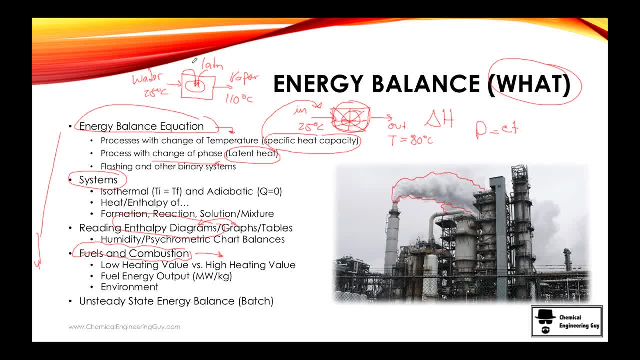 a change of phase. we want to understand how it happens and, more importantly, what is the change of enthalpy required now? eventually we're going to cover flashes and other binary systems, such as maybe a simple distillation column or, i don't know, a crystallizer, etc. and this unit operation. the good thing is that. 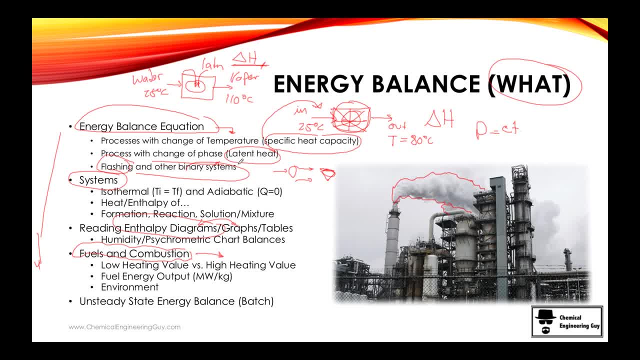 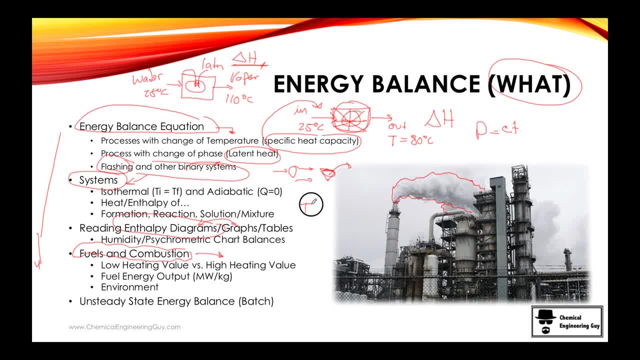 and what's an isothermal process? and yeah, probably you're probably telling me that if there is no temperature change, there is no heat or energy involved, and that is not always true. actually, latent heat, which is this one, is at one temperature. probably. you don't know, guys, but 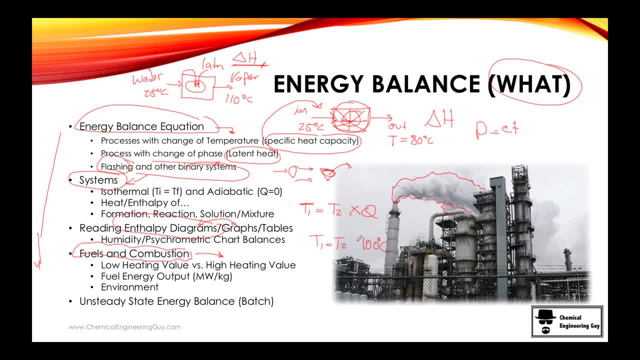 boiling water is carried out at 100 celsius, same temperature, but you do know that we need to keep boiling and boiling that water in order to convert it to vapor. everything at 100 celsius, and you will understand later that well, even though we don't have a temperature change, we may have a change on energy and also. 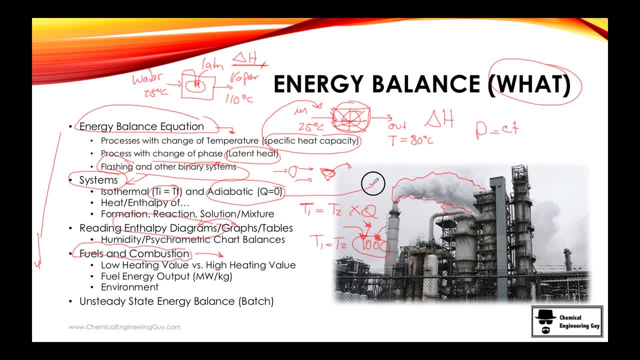 we will understand what's adiabatic and why are we so interested in adiabatic processes, especially when we want to change temperatures and involve other type of processes that favor adiabatic processes. now, guys, i told you about enthalpy, or typically heat off. they love saying the chemistry. guys love saying heat of formation. 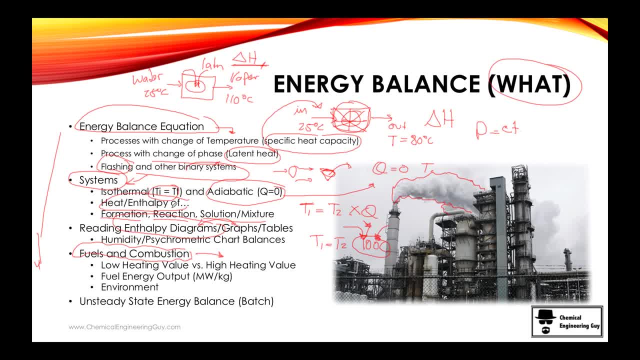 heat of reaction, heat of solution- well, that's actually only the enthalpy change of formation. so if i want to form carbon in solid state or co2 in gaseous state, how much enthalpy do i need? or how much heat will i need now for a reaction? the same if i want to produce b and there's a change of enthalpy here. 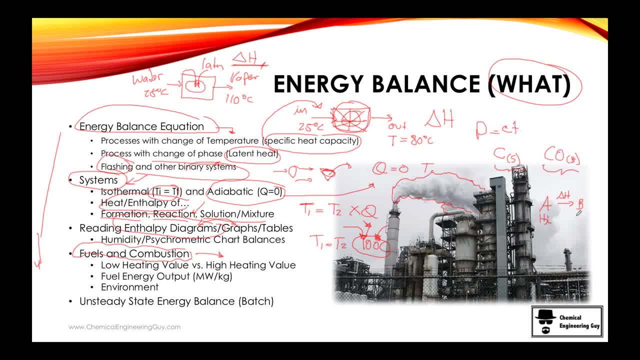 so i check out enthalpy, initial final enthalpy. i just need to make the difference and i got the change on enthalpy. that will be for a reaction, for a solution, exactly the same. i have a, i'm going to mix it with b, and they produce, let's say, well, a, b, and you know, guys, probably. 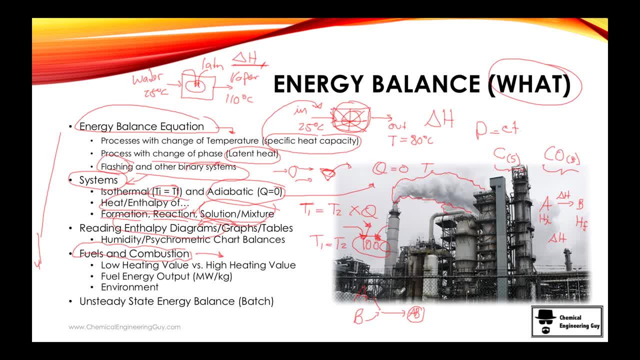 you're wondering: but where is the change of enthalpy? yeah, sometimes, when we mix substances, especially, let's say, water and ethanol, there is an increase of temperature. and why there's increase of temperature? because there is a change of enthalpy. now enthalpy: we've talked a lot of enthalpy, enthalpy. 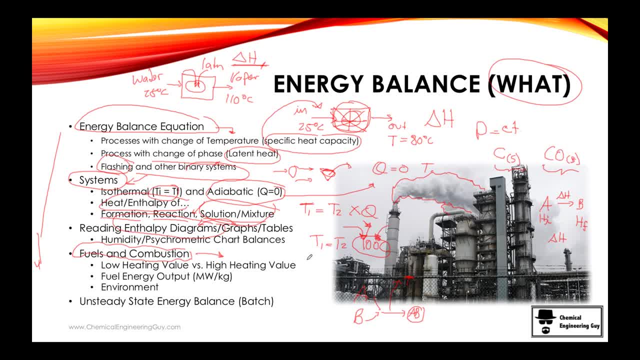 enthalpy. where can we find enthalpy? well, the first one is calculating it. you can change or calculate the change by raw calculations. it's a pain in the ass, yes, but eventually you get it and eventually you can start using graphs or diagrams. so plenty of students or researchers or scientists already. 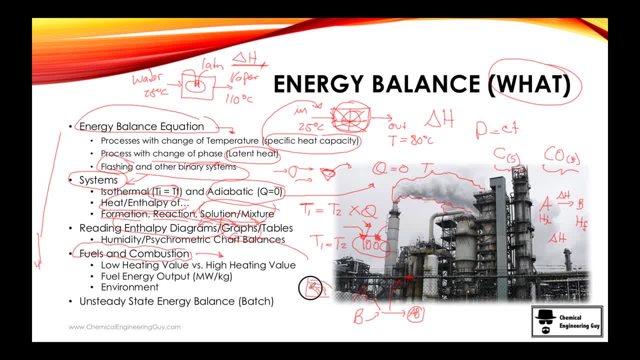 did what you do, which is essentially calculate all by hand all the changes. so you, instead of you actually calculating, you just check out for temperature and maybe you get a line right here and you got your enthalpy and eventually guys tables- we have the famous steam tables. 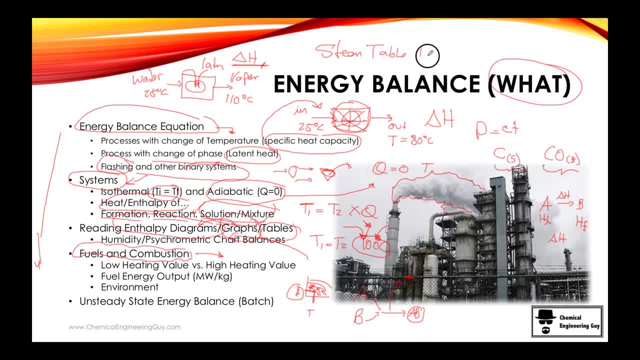 which carry a lot of information of water and vapor at many temperatures, many pressures, and has a lot of data. but let's just take care of the enthalpy right now. and once we've mastered how to do those calculations, we're going to work out on how to account for fuels, combustions, the famous low heating values, high heating values. 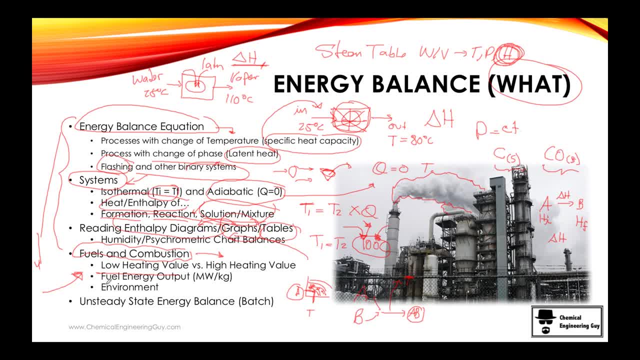 dry scale or humid fuel, etc. what's the energy output? and, of course, what's the environmental aspect of combustion or fuels. so, for instance, you can see this right here: what that is not good? probably co2, with other a little bit less sucks knocks, but plenty of co2. 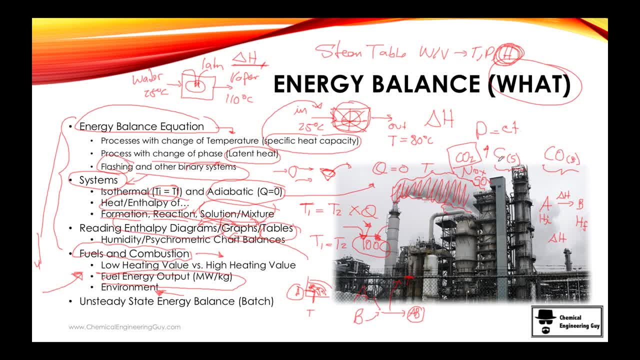 which you know is increases the temperature of the earth, which favors global warming. and finally, we do some unsteady states, because all this previously was done on steady states and you can see that there is continuous flow of these processes, such as this one, as you can see. 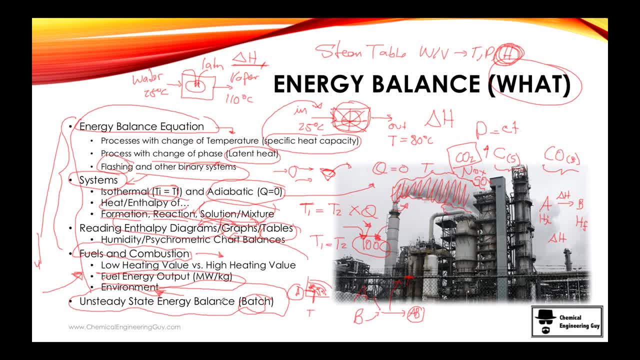 there is continuous flow of this smoke, but in unsteady states means batch processes such as: maybe you have this tank, you have water, you go burn it up and it goes out as vapor, and maybe you're going to use that vapor later on in order to- i don't know- heat something you're going to pass. 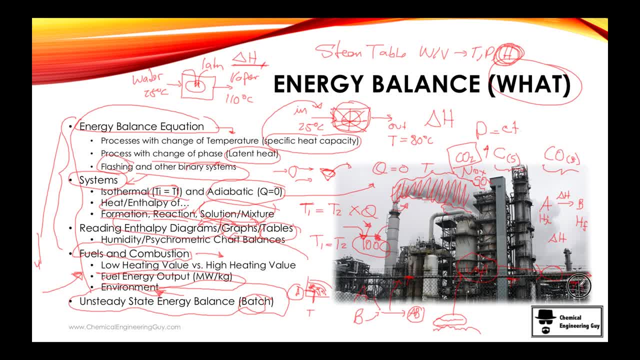 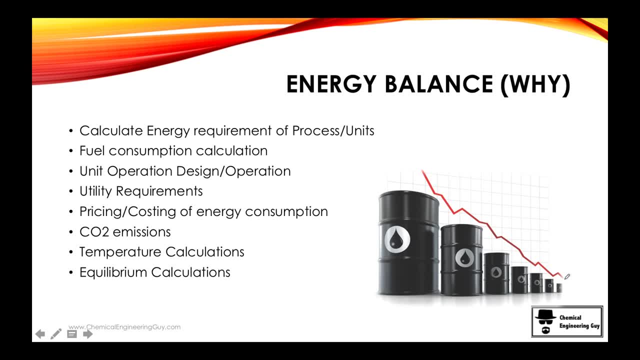 it through and high temperature vapor will go on unload and you're going to use that vapor later on and you're going to use that vapor later on and you're going to use that vapor later on. that was the. what do you see? now, the why of energy balance is essentially because we need to care. 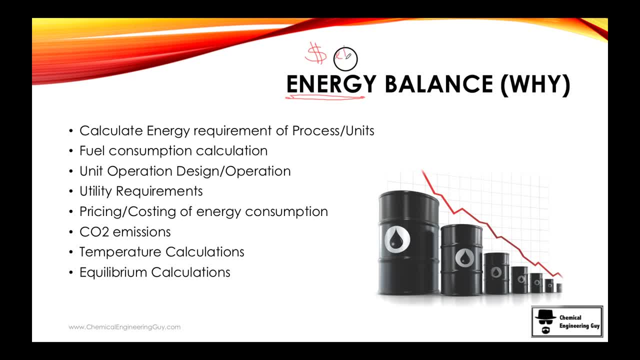 about energy. energy is expensive, guys. you know. the electricity or maybe heat or cooling down costs money. so it will be nice if we can maximize and optimize energy like this. so we're going to start doing some co2 analysis and we're going to start doing some co2 analysis and we're going to start doing some. 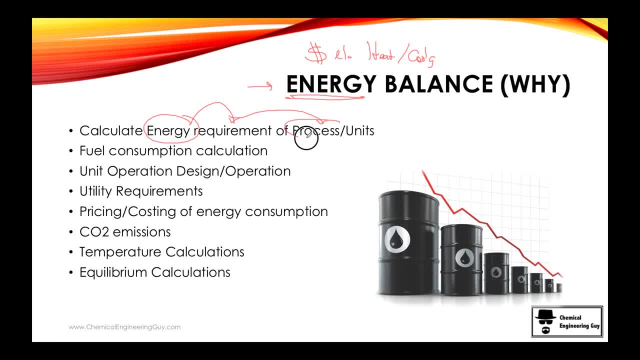 calculations on energy requirements for a process. for instance, let's say how to produce ammonia. well, the typical, i don't know. you need x amount of co2 per kilogram product, or maybe you need x, let's say y- amount of kilowatts per kilogram of ammonia. 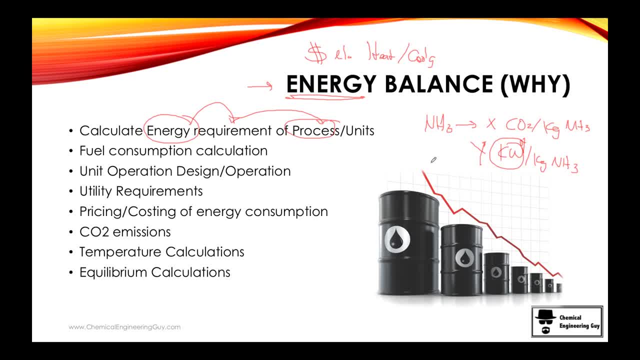 i thought this would be higher, very high number. uh yeah, we are interested in how much energy we need per process or maybe even unit. how much does that unit heating unit needs per time? so that's why we have a lot of kilowatts. maybe you check out in your light bulb you will see this is 80 kilowatt. 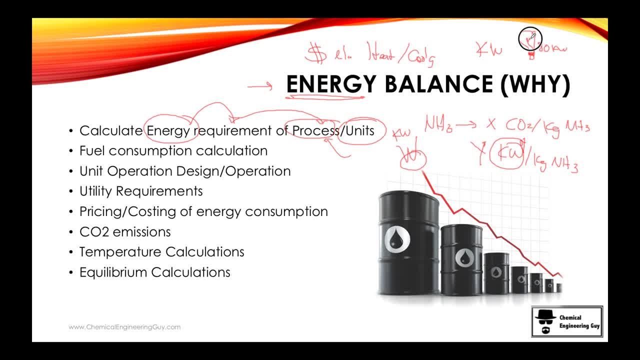 what does that mean is how much energy it requires in order to operate, give light, but of course it's also getting warm. so we have two time of two types or even three types of energy there. of course we have two types of energy there. now we want to calculate also fuel consumption. how much fuel? 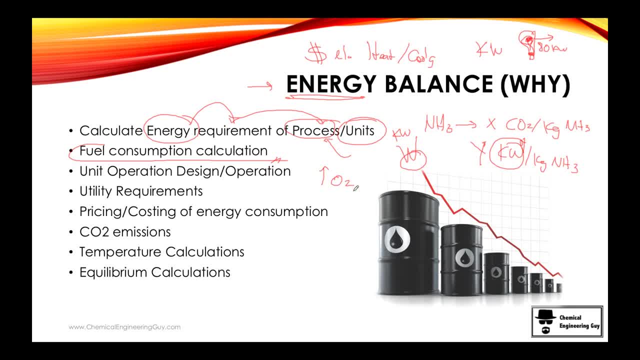 and especially if you are doing optimizations, if we increase oxygen or if we decrease, maybe, temperature or typically, you will also increase the temperature to increase the yield or conversion. also, it's needed because we need to know if it's possible if i tell you that we need a very huge condenser for a distillation column that is working with only 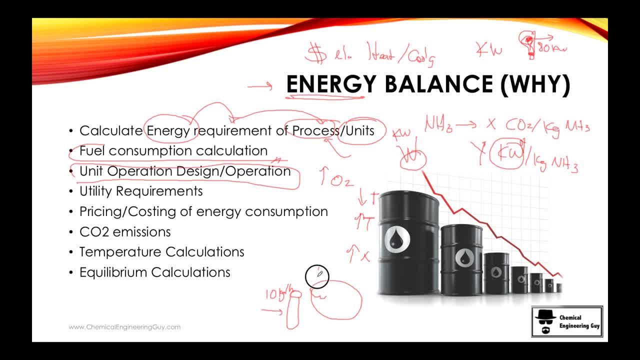 10 kilograms per hour, but we need, i don't know, maybe something stupid, let's say, 10, almost one ton of water per hour. so is it worth it? you need 10 kilogram of cooling water to work with 10 kilogram of feed. well, that's also interesting, and once again, it's the same. 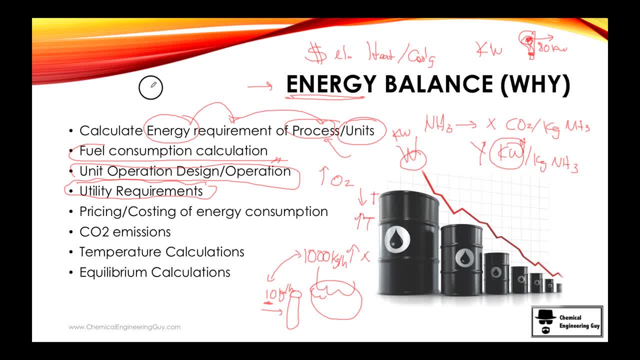 utility requirements. how much water do you need? how much air? because you're going to use air in order to cool stuff, those fans you have at your home. well, guys, we also have fans at the industry and they are huge and they give air. air cools down stuff. now we want also to make an analysis. 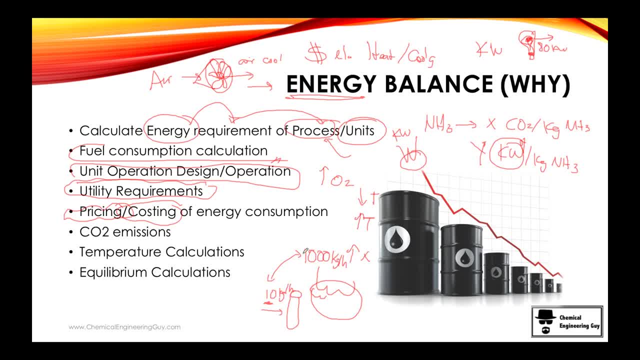 of cost. how much is the energy consumption in a plant unit in a country? maybe even also very important, how much CO2 burning? I think about 80% is fuel from fossils, so all that goes to co2. so if I want to hit 10 kilowatt, that will be a very interesting question. how much grams? 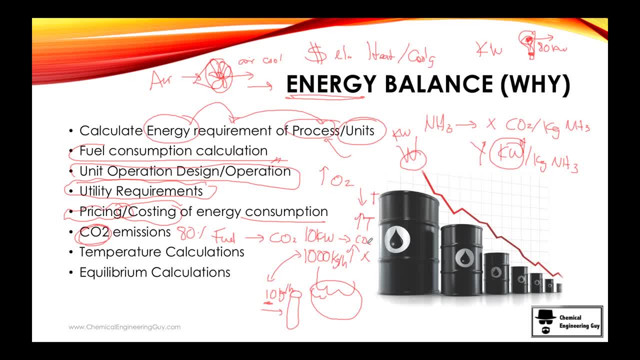 of co2 are we burning nowadays in USA or Mexico, Africa or whatever place you are. check out how much is that worth. maybe in a very, in a very good place you will have. you need three grams of co2, which I think is not that much, but maybe in not. 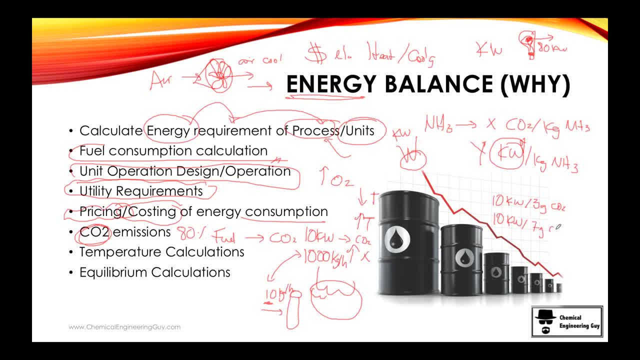 developed country, you will need- I don't know- maybe seven grams of co2, which means that you need probably 10 grams of fuel, and this will be about maybe five grams fuel anyway. finally, we want and we are very interested on temperature. heat, of course, relates somehow to temperature. so if we are interested in a 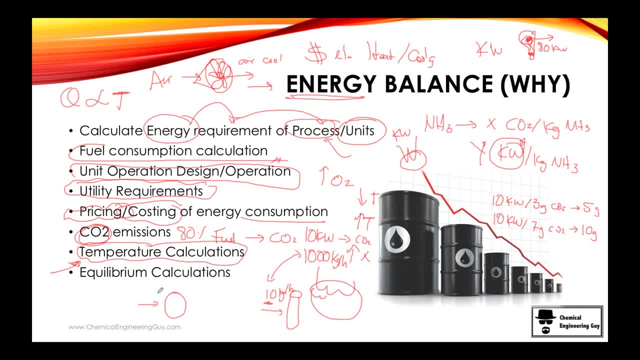 process. maybe if I tell you: I got this flash separator and I need it at 75 Celsius, but we got the stream at 30 Celsius. well, you're going to need to heat it. how much heat do we need in order to get that temperature? and finally, 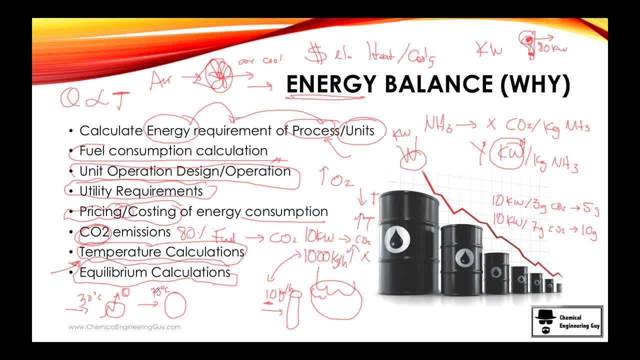 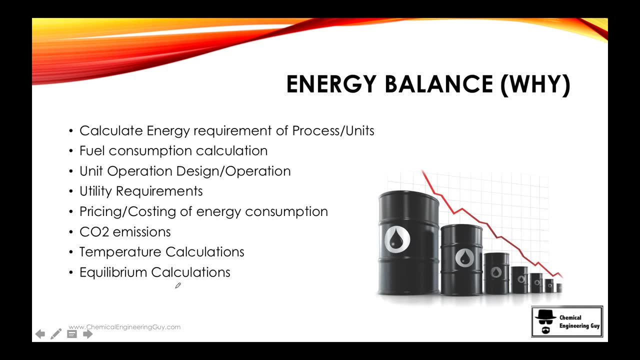 equilibrium calculations. not only we are interested: how much heat do we require? the question will be: how much are we going to separate if we achieve this temperature right here, and that's what I want to show you guys. energy balance, I will say, is a very basic course. I will say this: every process, process and you should take it. 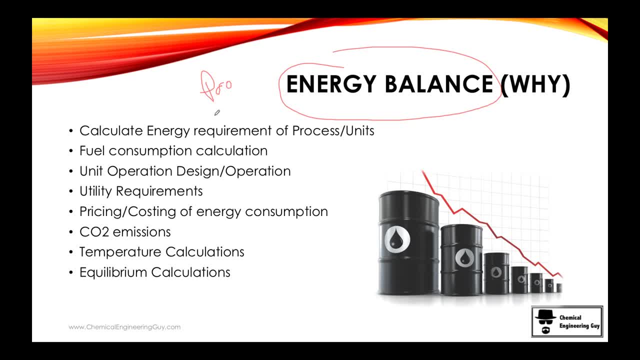 mechanical engineers, electrical engineers, maybe even software engineers, so they get to know how much energy they are spending when they're doing their engineering stuff. maybe- I don't know those servers guys that you think you're not- maybe you say using a computer doesn't waste that much energy. yes, it. 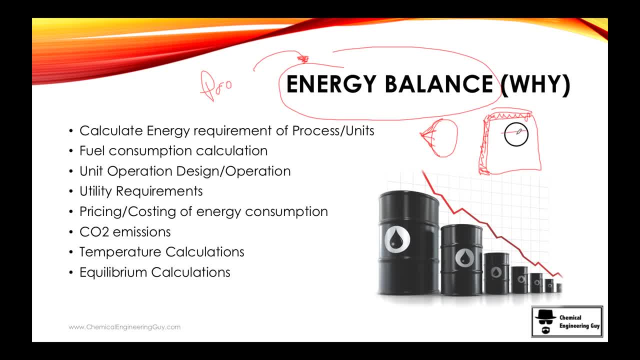 does, because internet needs of servers, huge servers- that because they work with electricity, by nature they give up heat and we need to cool those because if we achieve a temperature higher- I don't maybe 50 Celsius- it will start destroying our equipment, so we need to cool down that. so that was for energy. 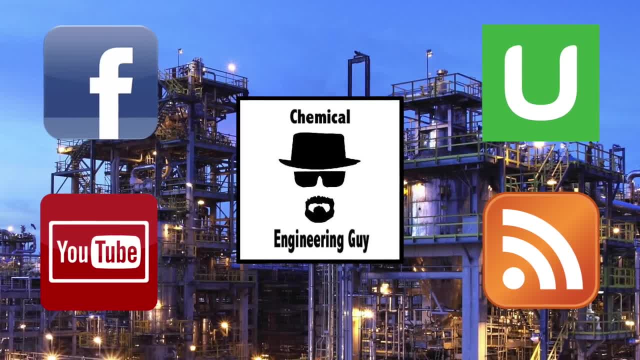 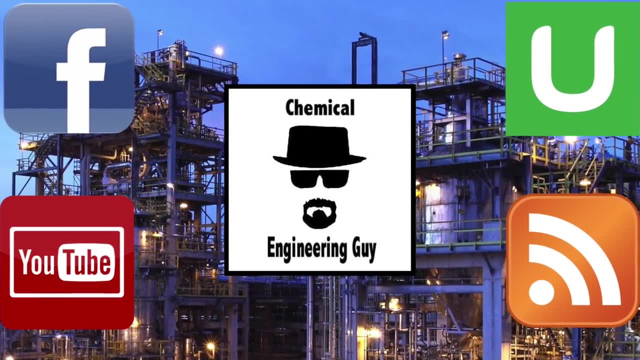 balance, then we go for thermodynamics. so we're going to go back to the thing that we talked about before. we are going to go back to the thing that we talked about before. we are going to go back to.